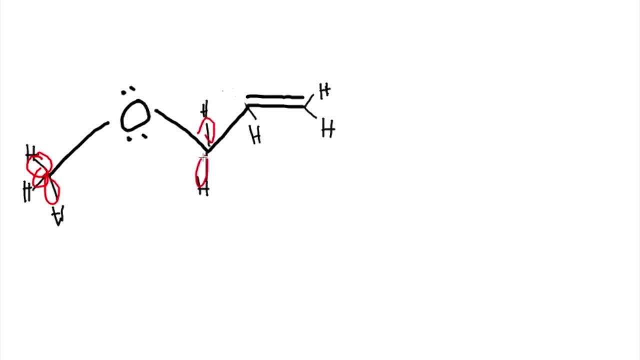 If there's any. So one, two, Three, four, five, six, seven, eight, nine, ten. The lone pairs don't count as sigma pi bonds. So there it is. in total, here We have ten sigma bonds. 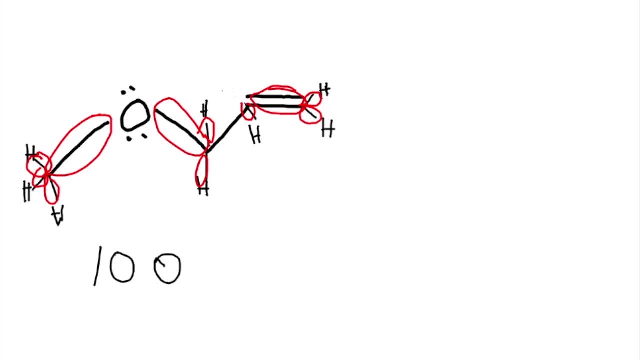 Now let's count the pi bonds, if there is any. So any double bonds. We have a double bond here, So this is only one. So we got one Pi bond here, Okay, So ten sigma bonds and one pi bond. So another example. 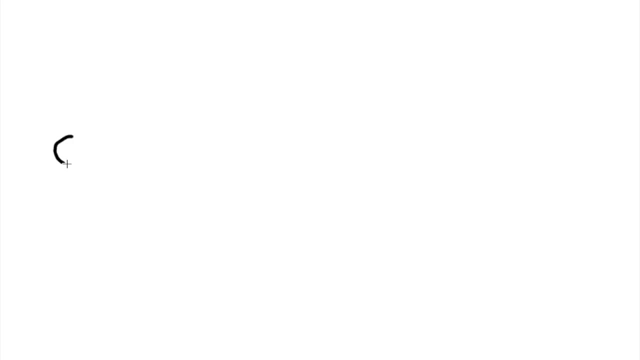 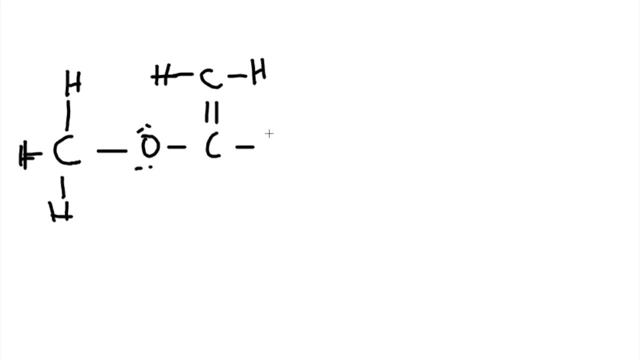